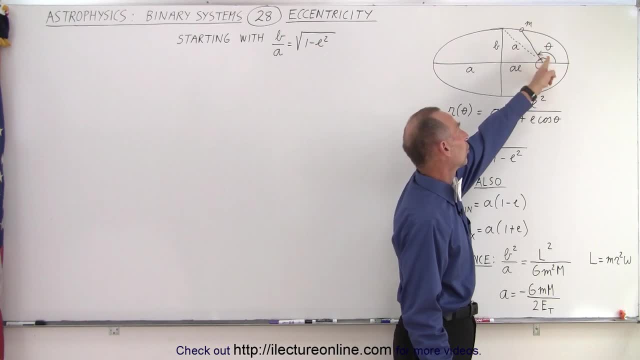 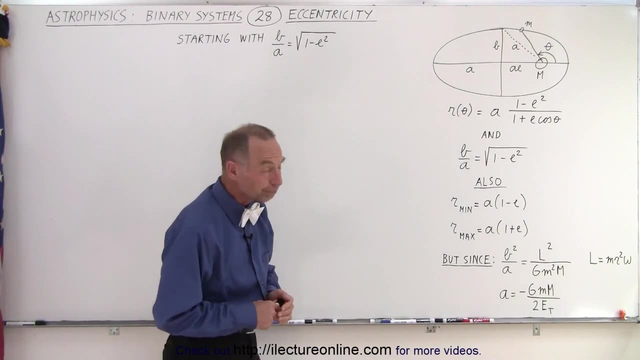 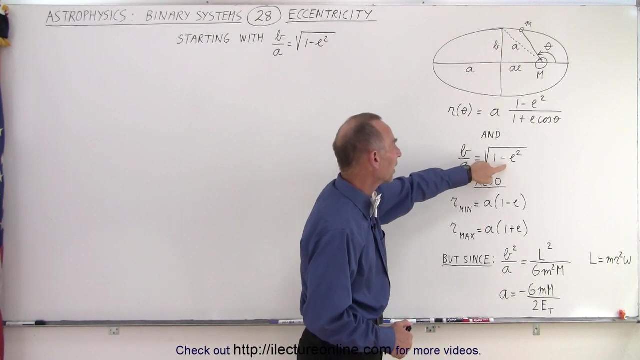 cosine of the angle theta, which is the angle of the horizontal axis to the position vector of the planet relative to the star or to the sun. Then we also know that the ratio of the semi-minor axis to the semi-major axis is equal to the square root of 1 minus e squared. 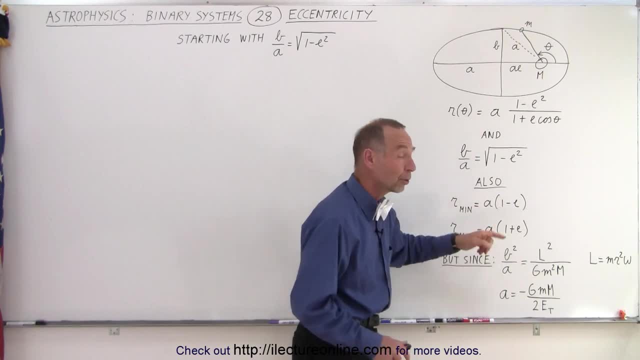 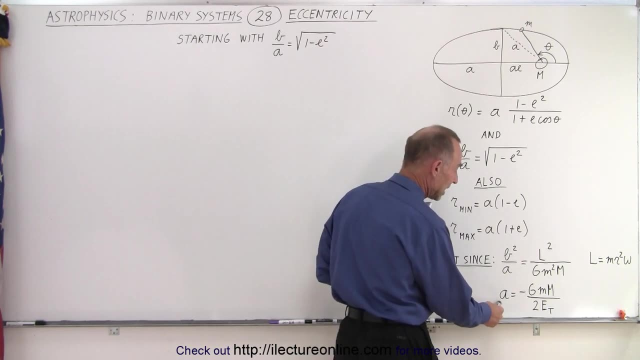 We can also write the eccentricity In these two equations, which is what I typically use. it's kind of easier to use these two equations. or we also know the relationship between A, the semi-major axis, and the properties of the two objects. the larger object, the smaller object, mass, We have the total energy. 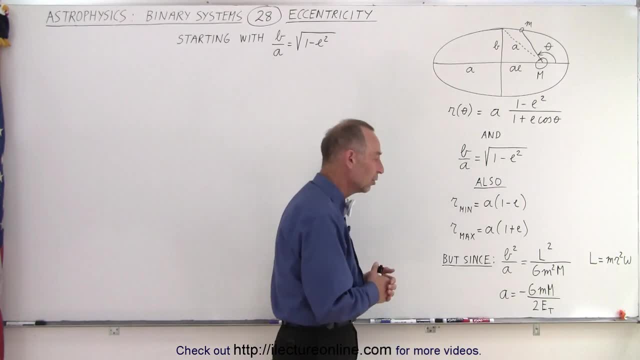 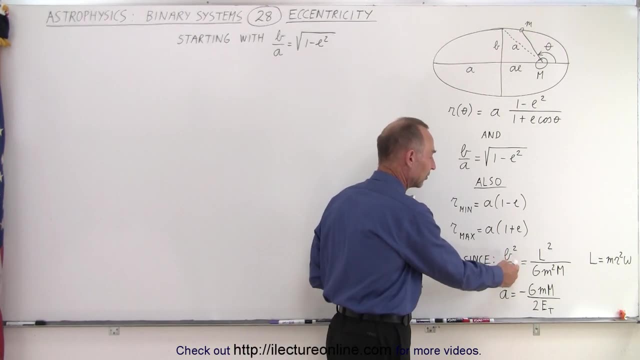 of the small object of the planet, and the g, which is the universal gravitational constant, and also the ratio of b squared over a, where b is the semi-minor axis and a is the major axis in terms of the angle of momentum. g, small m and large m. 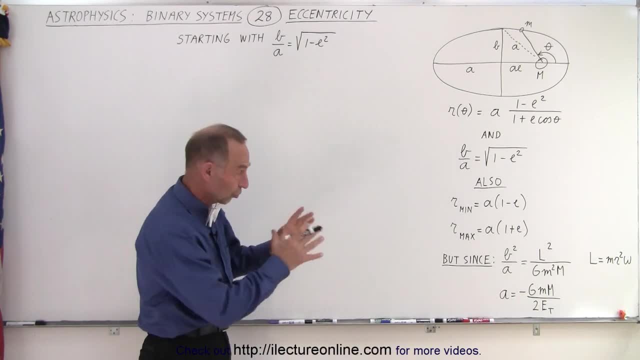 So we're going to go ahead and use those properties now, those relationships, to come up with an equation for the eccentricity that describes eccentricity in terms of the mass of the planet, the mass of the sun, the angle of momentum of the planet and also the total energy of 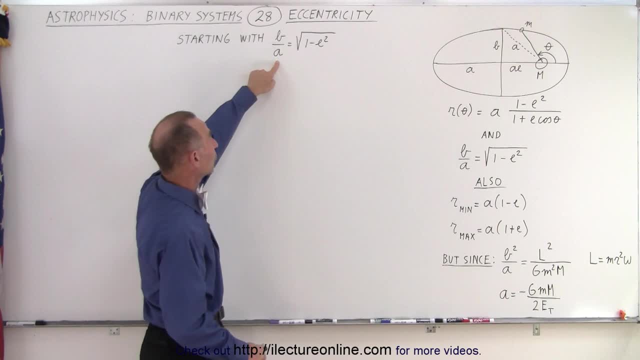 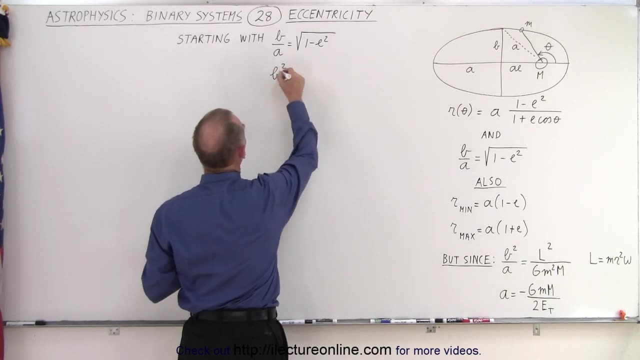 the planet. So we'll see how we can derive that. So we're going to start with this equation right here, which is the same as this equation right there. Now we're going to square both sides. so when we do that, we get b squared. 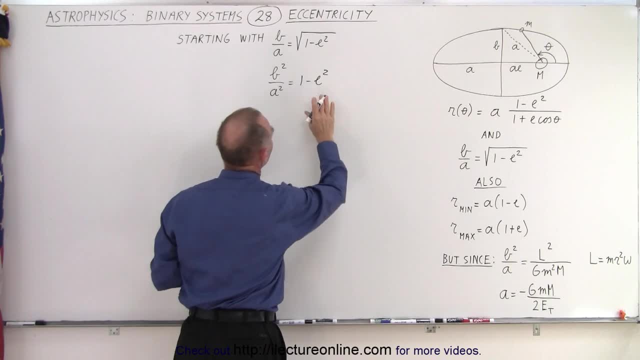 over a squared is equal to one minus e squared. and then we solve this for e, the eccentricity. so we have: e squared is equal to one minus b squared over a squared. And since I have this relationship right here, we're going to write this as one minus b squared over. 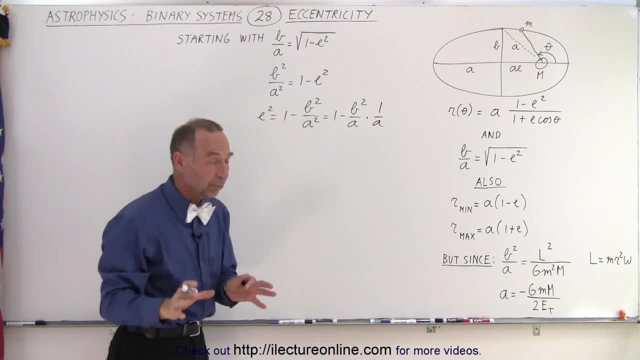 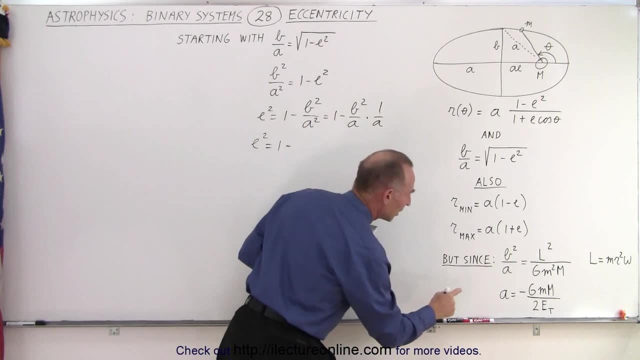 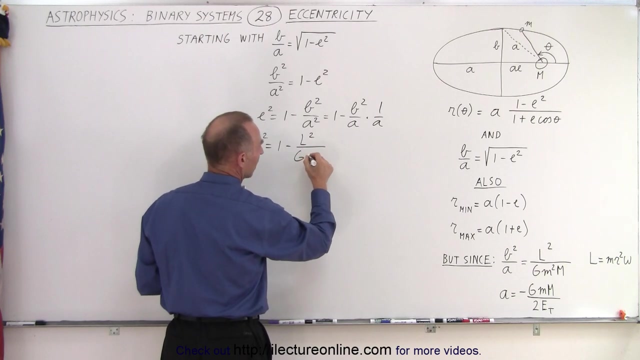 a times one over a, And now we're going to substitute what these two fractions are equal to. So now we have: E squared is equal to 1 minus, so B squared is defined right here. so that is equal to L squared divided by G: small m squared big M. 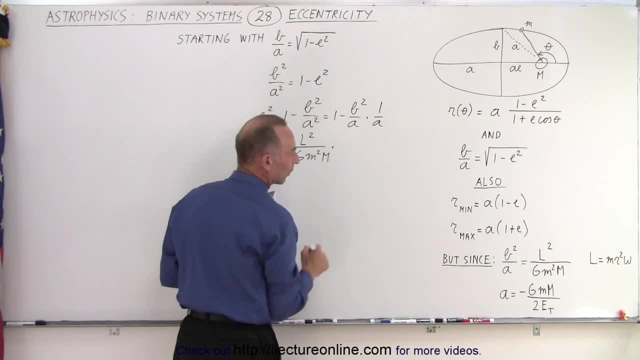 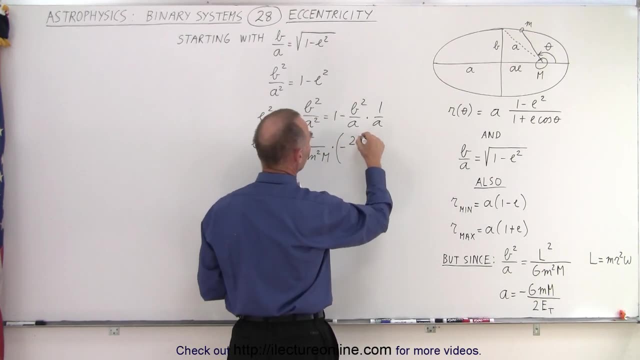 so that's the mass of the planet, the mass of the sun, times 1 over A. Now, of course, A is equal to this, so 1 over A will be the inverse of that. So we need a minus sign. We have twice the total energy divided by G, m, big M.